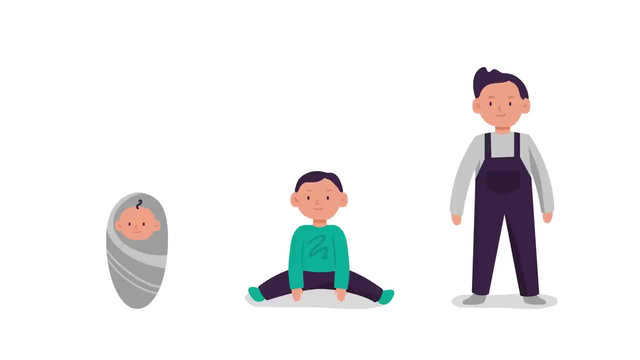 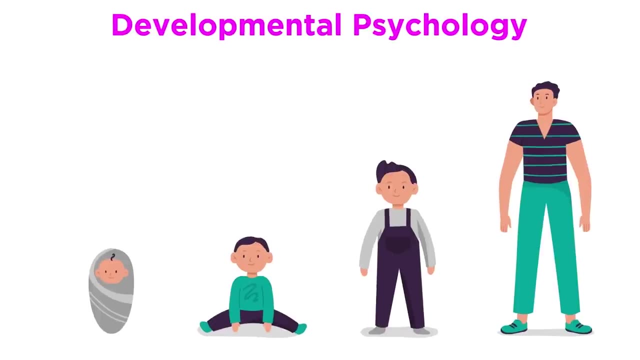 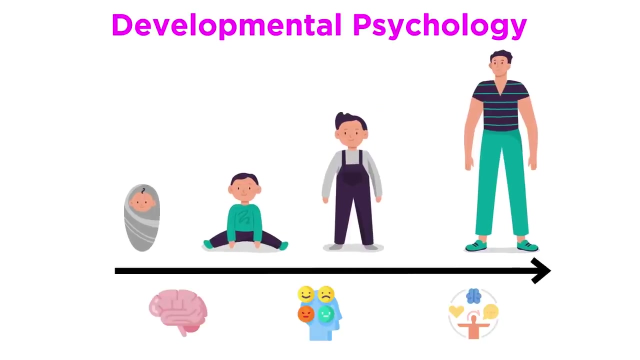 and what happens during this time period can have a lasting impact on their behaviors in adulthood. The field of developmental psychology tries to explain how and why people's thoughts, feelings and behaviors change over their lifetime, with a particular emphasis on childhood, since this is when a lot of important changes occur and these changes predict later adult. 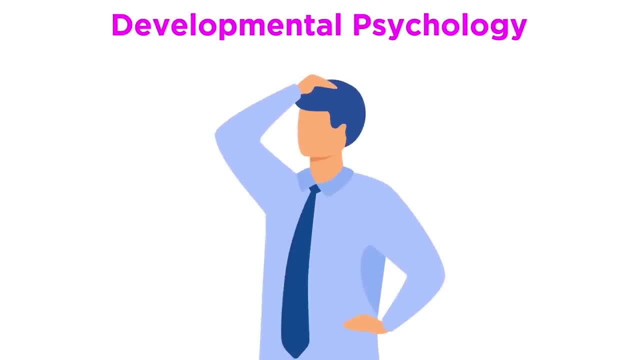 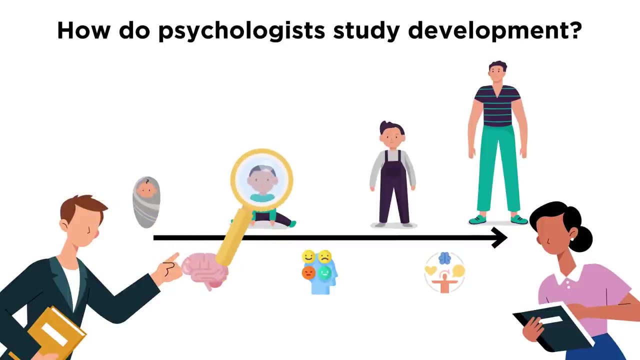 psychology. Developmental psychology is an enormous topic that would be impossible to cover in a single video, so let's simply hit some highlights. for now. Let's start with the basics. How do psychologists study development? Psychologists have a few different techniques to answer different questions. Let's say you're interested in 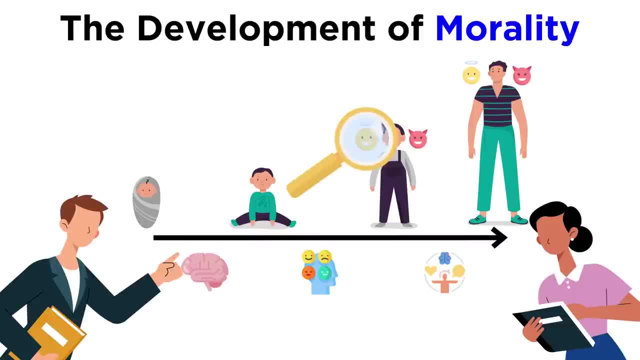 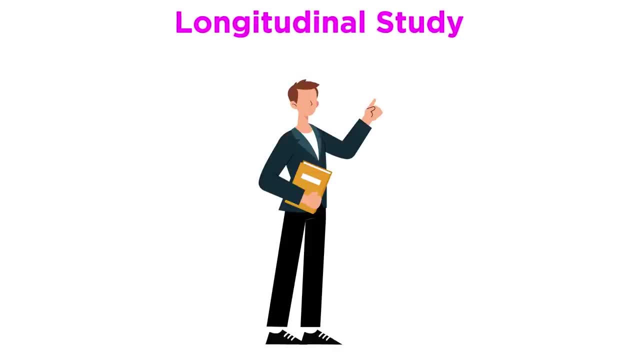 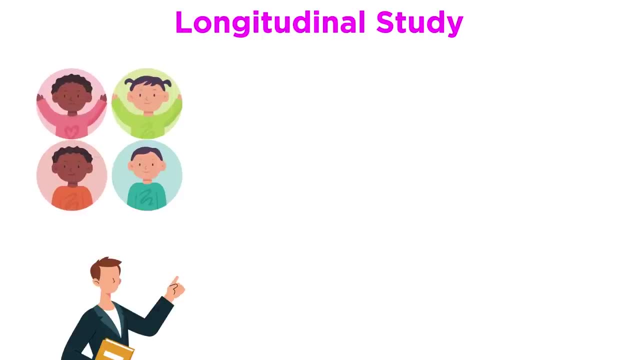 the development of morality. How does it change across one's lifetime and when does it develop? To answer the first question, you would want to perform a longitudinal study and follow the same group of people as they grow up. You would take a group of young children, say four-year-olds, and ask them what they think. 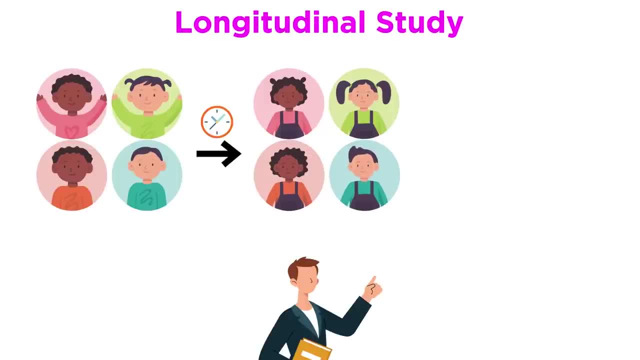 right and wrong means, Then you would bring them back into the lab every few years, ask them the same questions and see how their answers change. If you cared less about how morality changes across development and more about when children develop morality, you would. 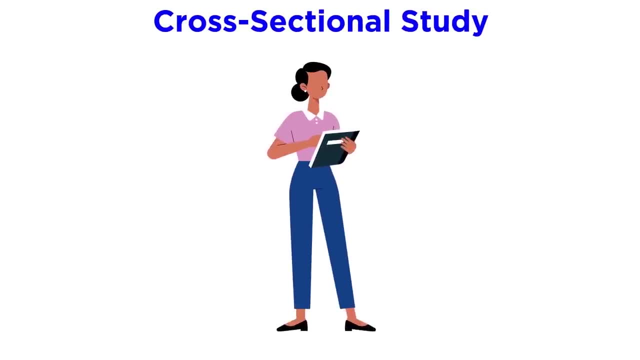 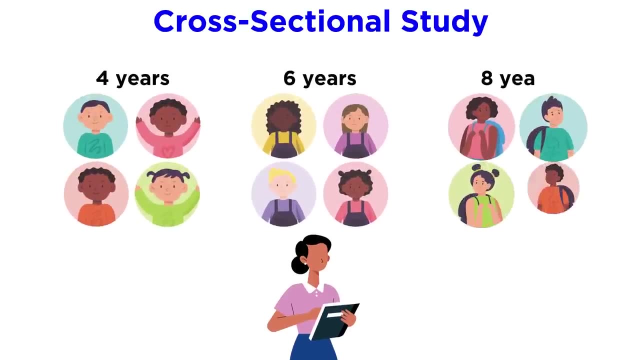 probably do a cross-sectional study or an age-of-onset study. For a cross-sectional study, you would take a group of young children and ask them what they think right and wrong means groups of kids at different ages- and see how their behaviors differ. How does the morality 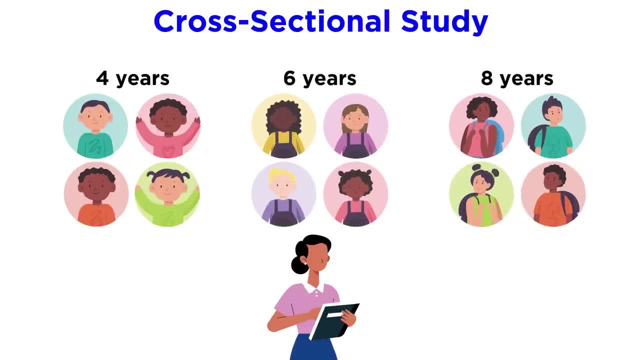 of eight-year-olds differ from that of six-year-olds and from that of four-year-olds. An age of onset study is similar in that you're studying different age groups, but in this case you don't compare the age groups to each other. Instead, you ask: what do four-year-olds do in? 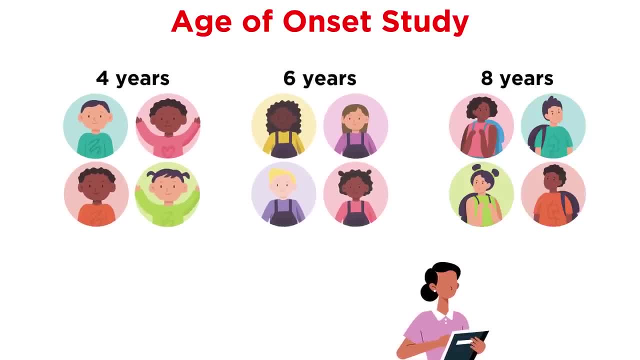 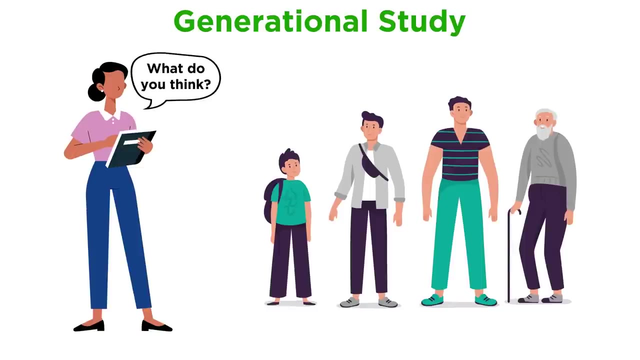 this morality task. What about six-year-olds? What about eight-year-olds? Finally, let's pretend you're interested in how growing up at different times might affect morality. You would do a generational or cohort study in this case, and ask how people who grew up in different times 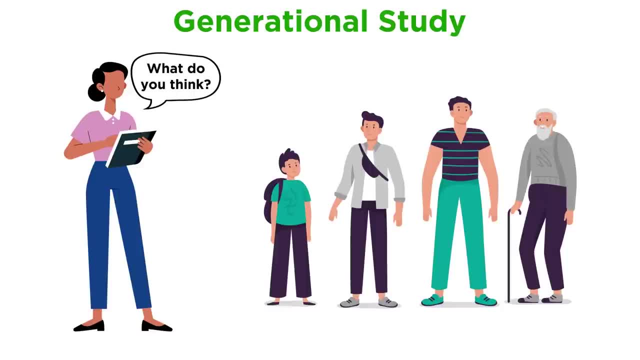 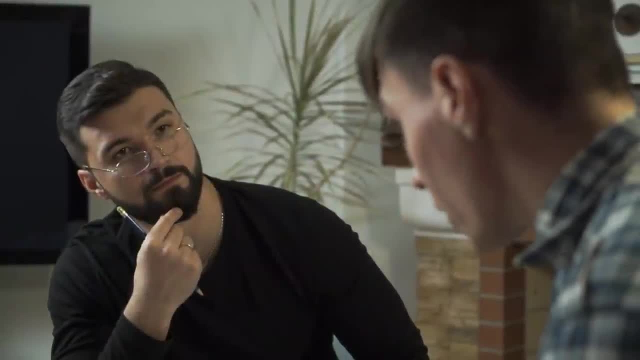 thought about morality. Do boomers have the same ideas about morality as millennials? If not, how are they different? Now that we have a basic understanding of how to grow up at different times, let's talk about how to grow up at different times. 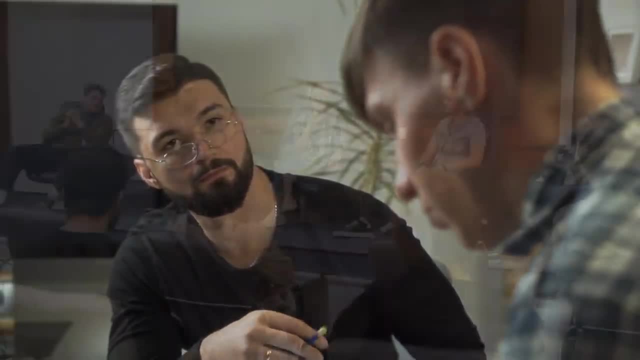 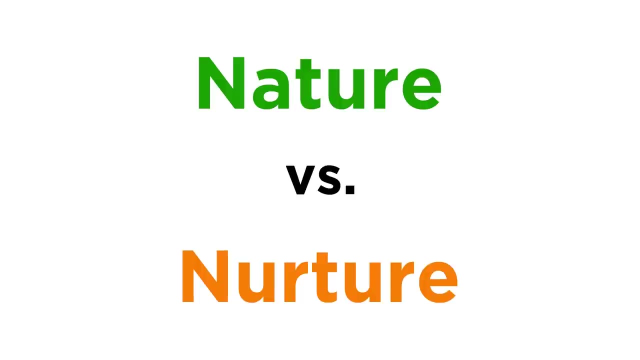 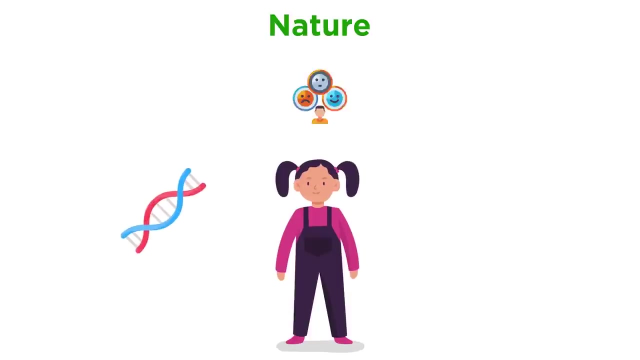 How developmental psychologists tackle developmental questions. Let's talk about a debate you may have heard of nature versus nurture. This debate is about what has the biggest influence on child development. Is your development constrained by nature, where the genes you possess control your behavior and psychology, Or is your development more? 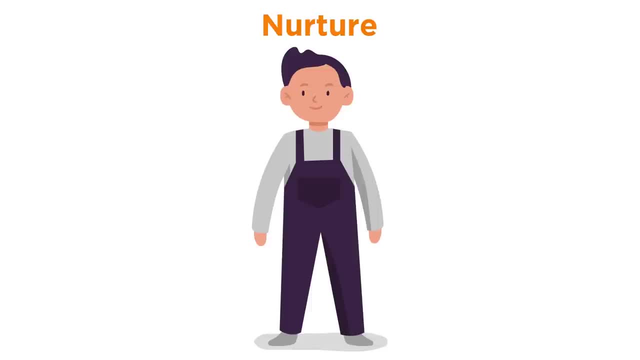 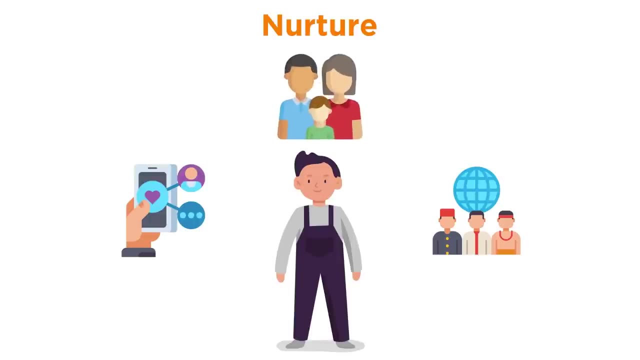 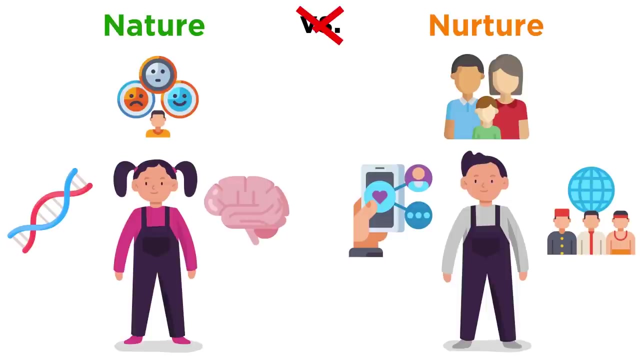 influenced by nurture, meaning everything else that could influence your behavior, like learned associations from experience, the social and cultural environment or your interactions with other people. Well, the answer is both. The idea of nature versus nurture is a false dichotomy. We don't have to pit nature and nurture against each other. 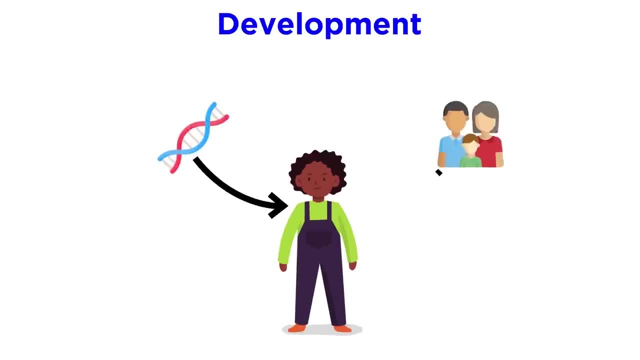 Development is influenced by both your genes and the environment you're in. In fact, your environment and social interactions can influence which genes are expressed and how they are expressed, ultimately affecting your behavior. While some behaviors may be more influenced by genes, they may not be influenced by your behavior. So let's talk about how you can. 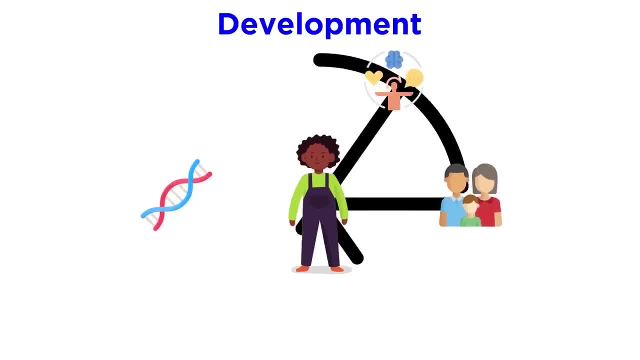 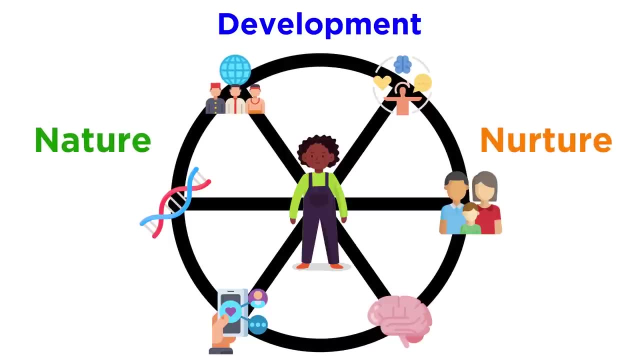 child development factors than others, and vice versa. Development as a whole is affected significantly by both nature, the genes you have, and nurture, the environment you're in. Let's move on to actually talking about kids and how they develop. An important thing to note is: 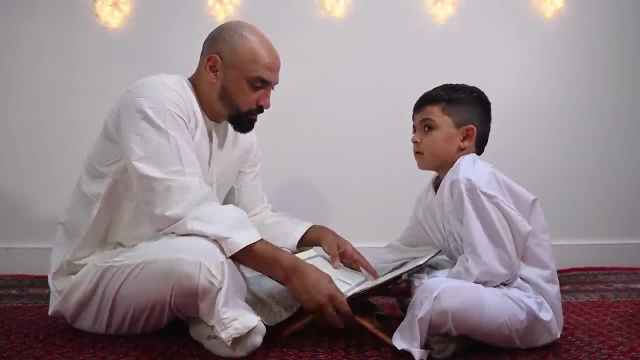 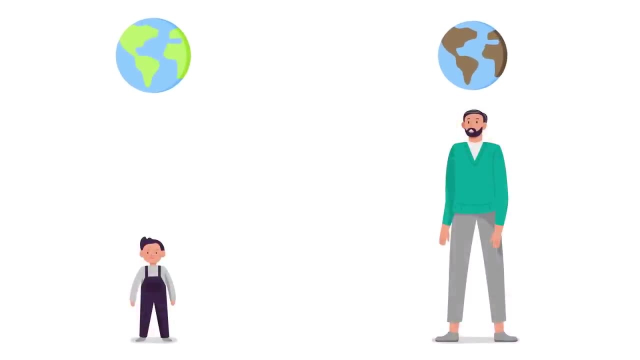 that children are not just really dumb adults. Children occupy a very specific developmental niche. The way they view and interact with the world is inherently different from adults and will change in the future. So let's talk about how they develop. change as the child grows and develops. 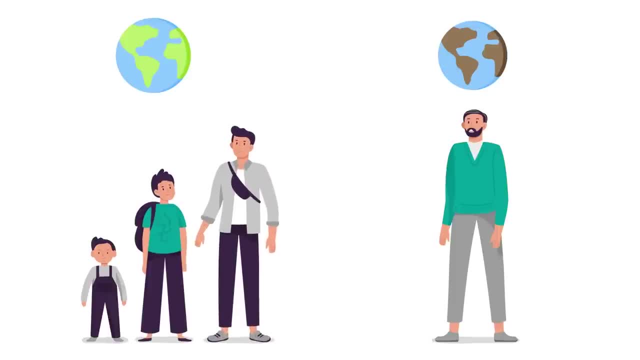 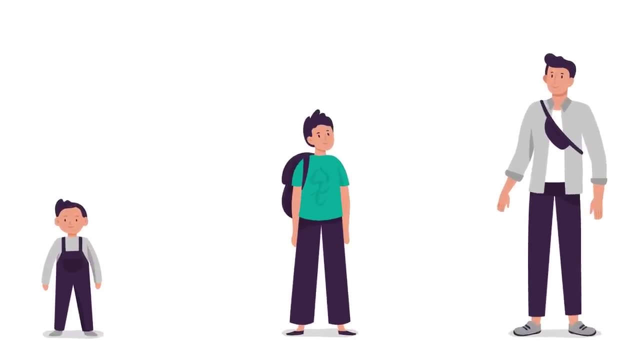 This means that kids think and reason differently than adults and will see the world in different ways. As a child grows, they build up their knowledge about the world through their experiences. They are actively experimenting with the world around them and from the results building. 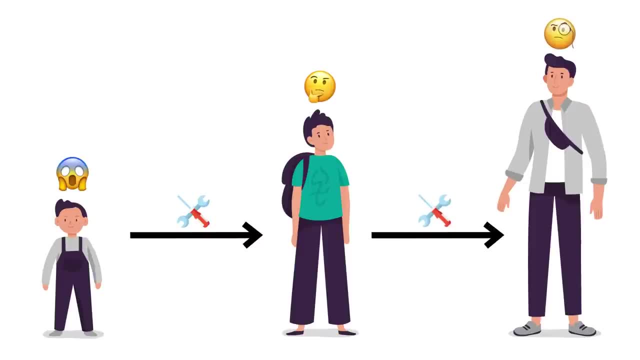 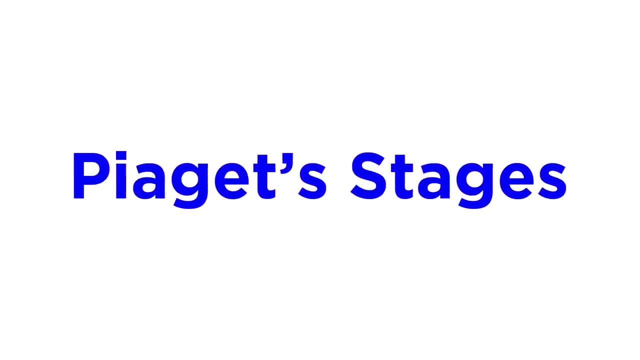 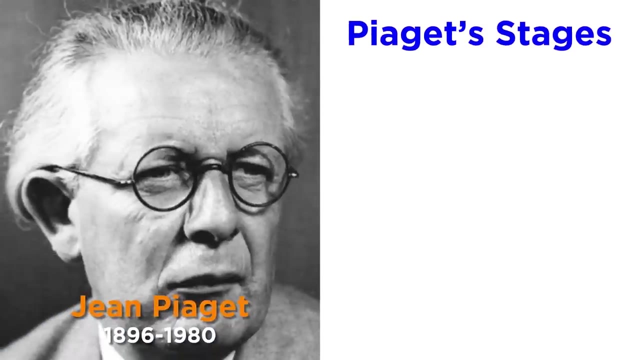 an understanding of how the world works. To get a framework around this process, we are going to focus on a theory that is commonly used to describe child development, known as Piaget's Stages. Jean Piaget was a psychologist in the early 1900s who proposed a theory to describe how 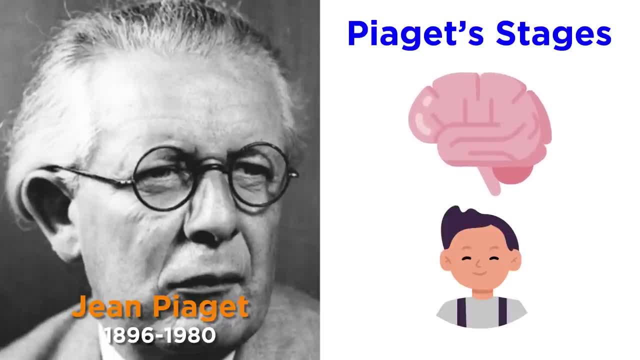 children's intelligence grows and changes. His theory relies on the idea that cognitive abilities build upon one another As we go through these stages. we will reference some approximate ages at which children go through a particular stage. Adults today generally think that all children go through these stages in this order, and 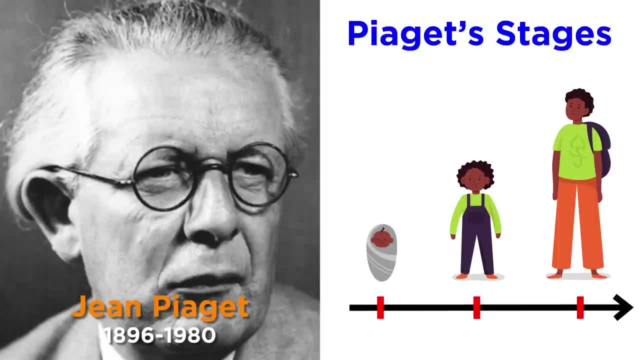 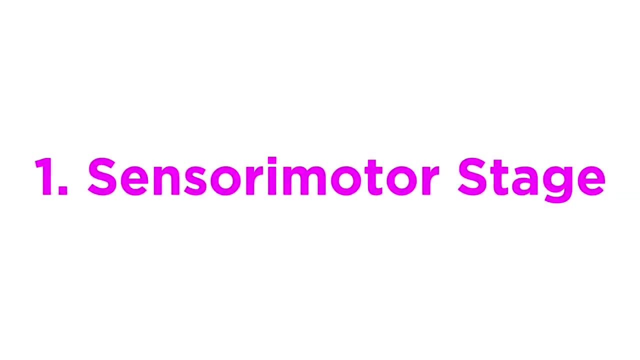 on average at these time periods, but there is some variation. Certain kids move through the stages faster than others, and these kids aren't necessarily smarter. it's just some natural variation. Let's move through Piaget's stages now. The first stage is called the sensory motor stage and this usually occurs between birth. 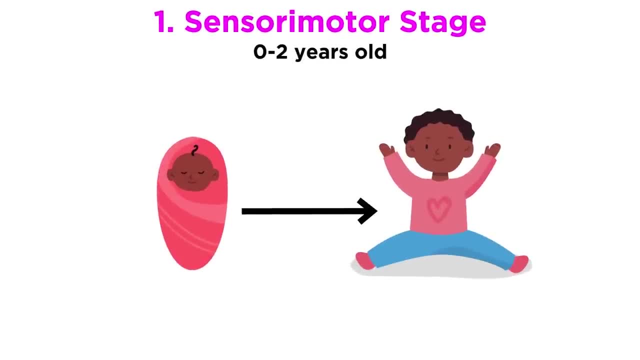 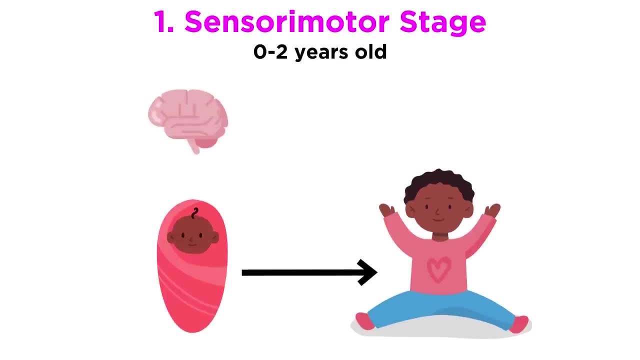 and two years old. This stage is characterized by the sensory motor. It is characterized by an enormous amount of growth and learning. We all go from being an infant who is lightly interacting with their world through reflexes to a toddler who is actively moving and exploring. 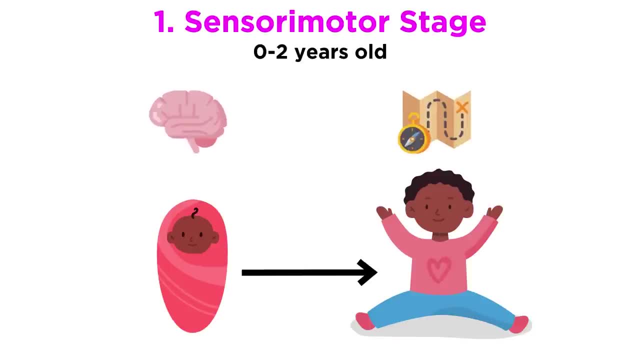 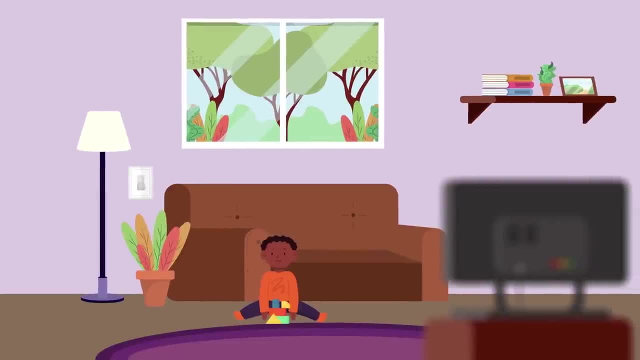 Kids in this stage use the skills and abilities that they are born with, like looking, grasping and listening, to explore their environment. They use their senses and motor abilities to learn through trial and error about the world around them. It's during the sensory-motor stage that children are born. 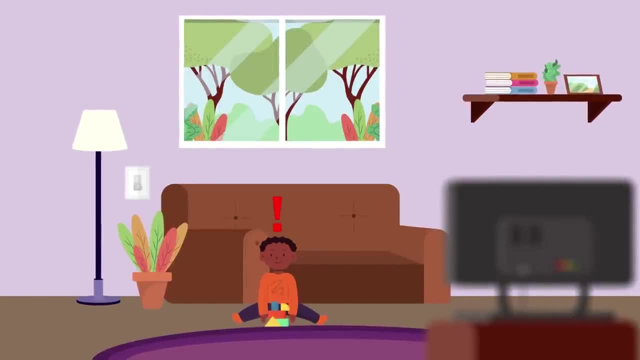 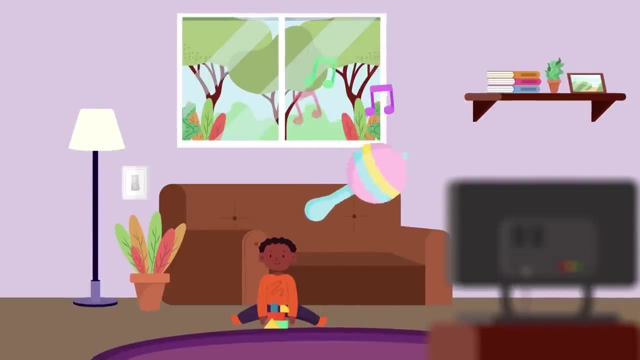 It's during the sensory-motor stage that children begin to learn that their actions can cause specific reactions. For example, they might begin to realize that when they shake a rattle it makes a pleasing sound, Or that pushing a light switch causes a light to turn on or off. 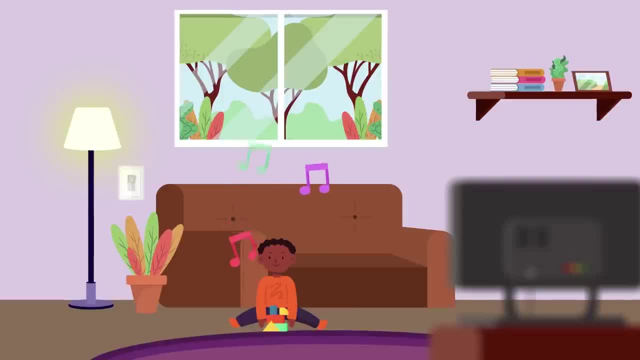 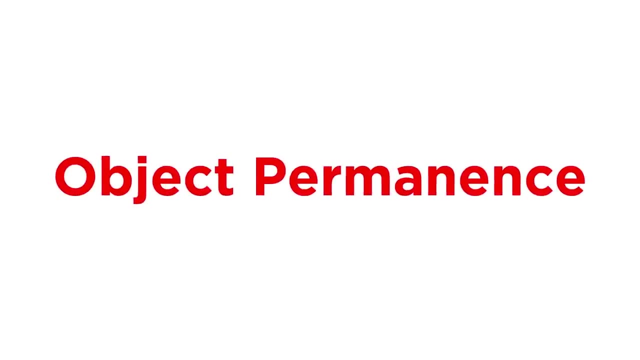 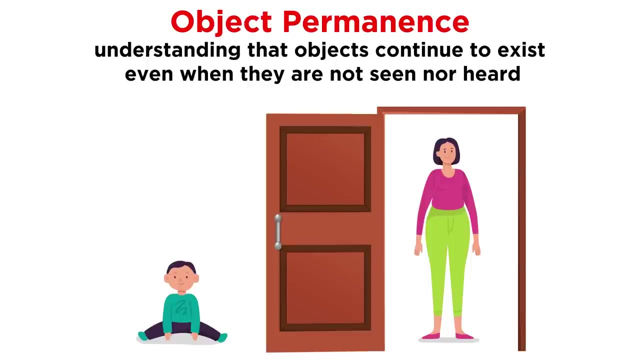 They also might try to make different sounds to see if they can get a response from a caregiver. An important cognitive milestone in this stage is the development of object permanence. Very young infants do not have object permanence, that is, they don't understand that objects. 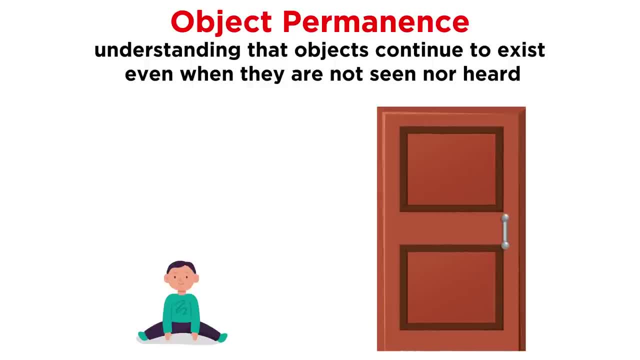 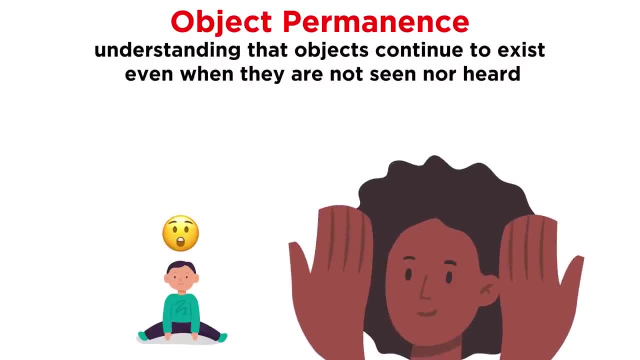 continue to exist, even when they can't be seen or heard. This is why young infants will act surprised during a game of peek-a-boo. When you hide behind your hands, the infants believe that you are actually disappearing. Older infants that have developed object permanence will learn and understand that you continue. 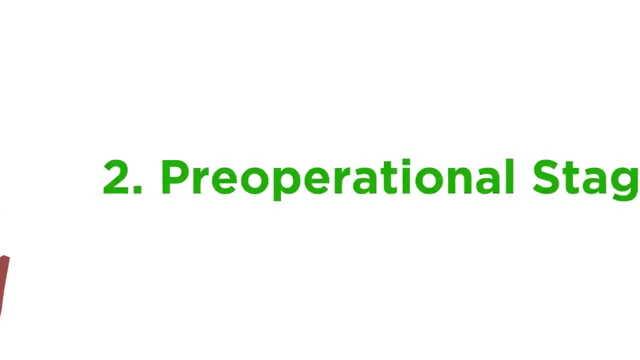 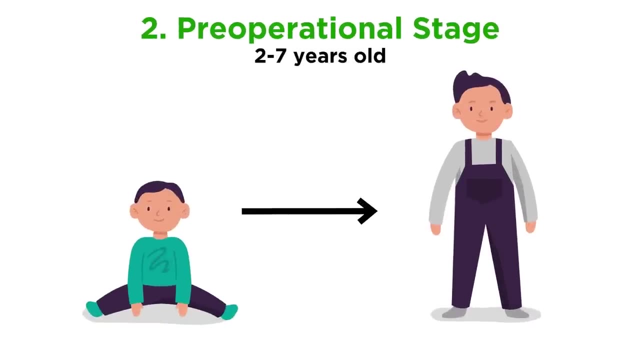 to exist even when they can't see you. The next stage is the development of object permanence. The next stage is the pre-operational stage, which happens around two years old to seven years old. In this stage, children become proficient in language. 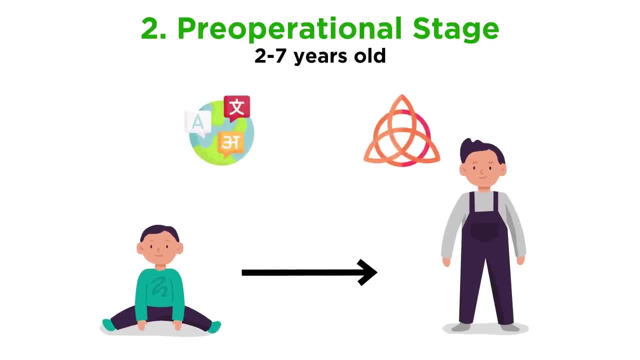 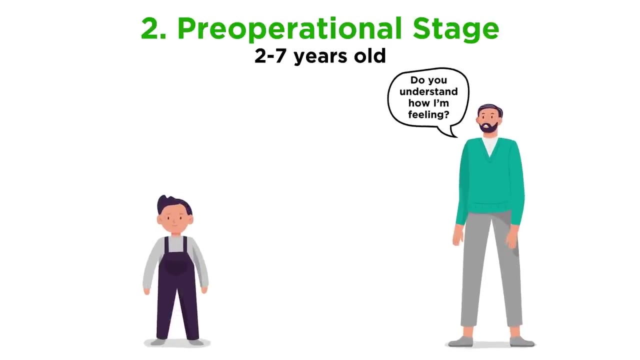 They also begin to think symbolically. as you know, if you've ever played pretend with a child, They can use an object to represent something else, like pretending a broom is a horse if they want to be riding a horse. Kids in this stage still struggle with some logical tasks and often struggle with adopting. 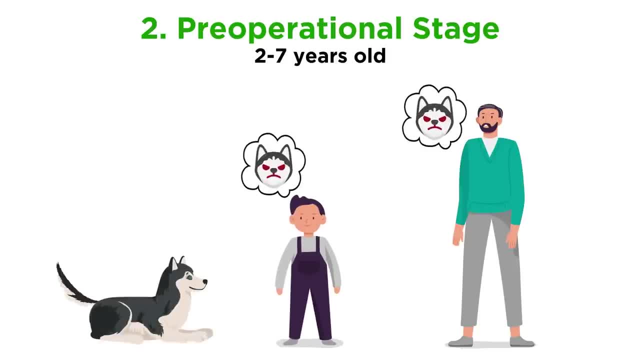 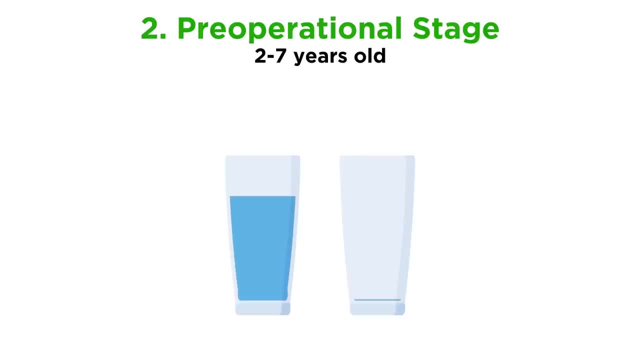 a view of other people. They may think that everyone sees things as they see them. They also struggle with conservation. For example, say you have two identical containers with equal amounts of liquid. Then you pour the liquid from one container into a differently shaped cup, like a tall. 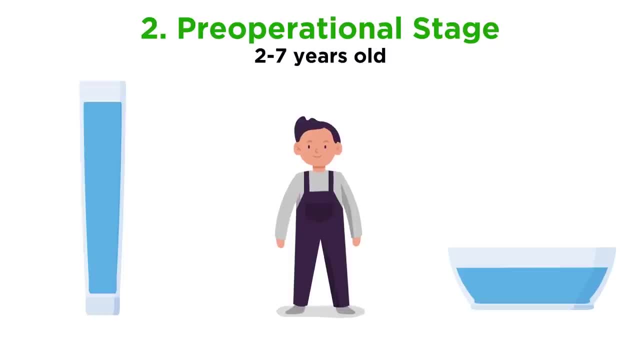 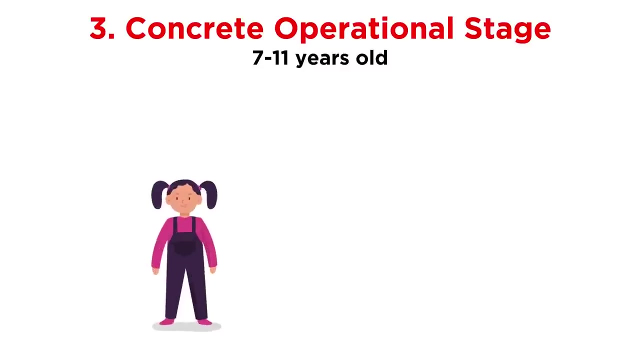 thin cup or a short wide cup, Even though the amount of liquid did not change. children will say that there is more liquid in whichever cup appears to be fuller. The third stage is the concrete operational stage, which takes place between around seven and eleven years old. 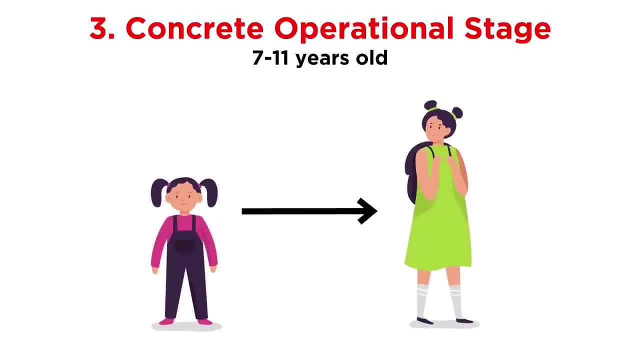 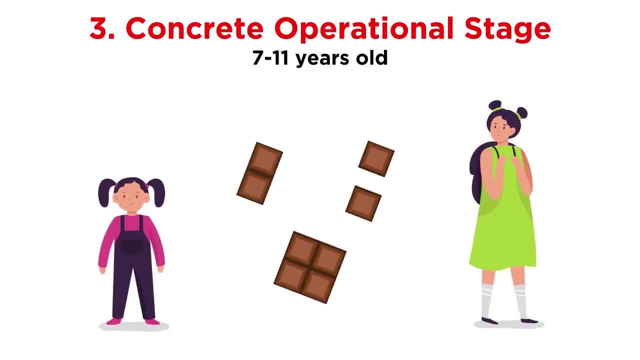 Unlike in the previous stage, children now understand conservation. They know that breaking a candy bar into more pieces does not mean there is more candy. Children in this stage also begin to develop logical thought. Although they still tend to be very concrete in their thinking, children are beginning. 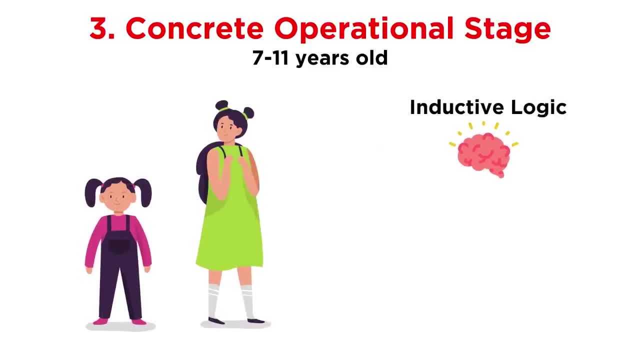 to excel at certain logical tasks like inductive logic. This means that they can go from a specific experience to a general principle. Say, you notice that every time you're around a cat you get itchy eyes and a runny nose. Children who have mastered inductive logic would then be able to induce that you are. 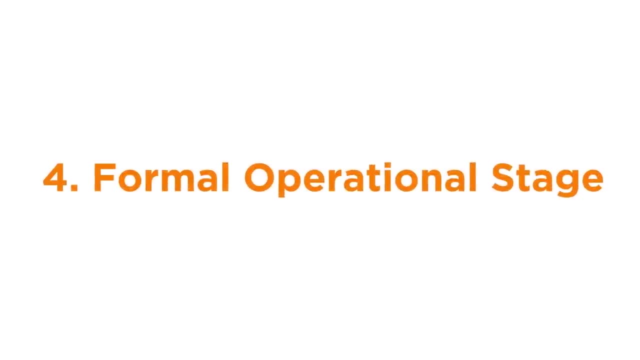 allergic to cats. The fourth and final stage of Piaget's stages is the formal operational stage, occurring when kids are around twelve years old and older. This means that they can go from a specific experience to a general principle. This means that they can go from a specific experience to a general principle. 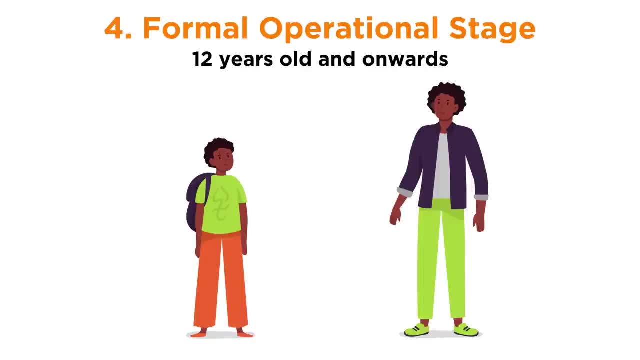 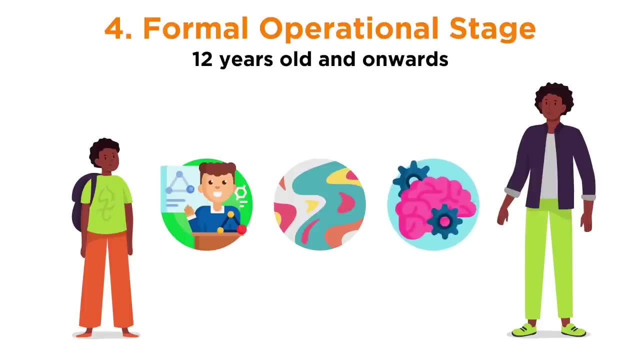 Children and adults in this stage have the capacity for much more sophisticated thought. They can think about abstract and theoretical concepts and can come up with creative solutions to problems using logic. In this stage a child doesn't need actual, concrete objects to answer questions via trial. 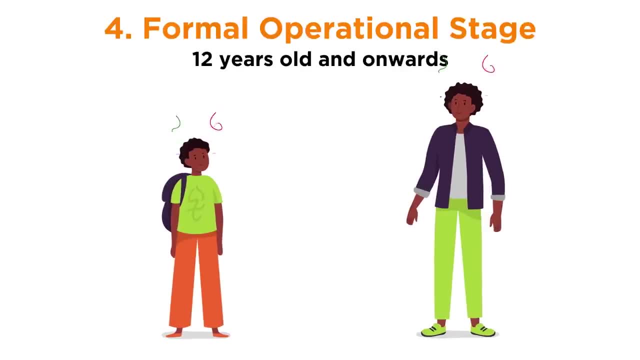 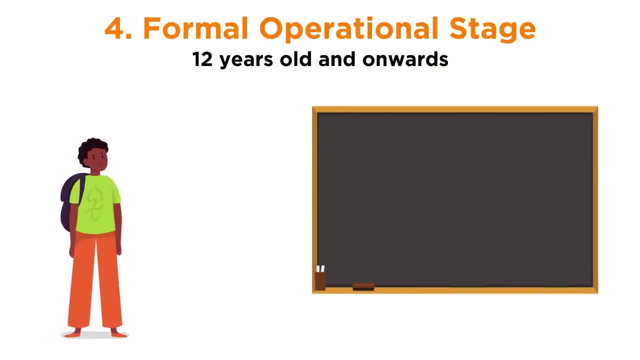 and error. Instead, they can perform mental operations in the head using abstract terms. For example, kids at this stage can work through the following question in their head: If you imagine something made up of two quantities and the whole thing remains the same when 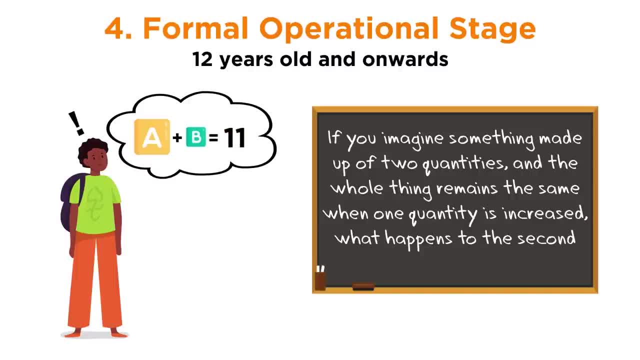 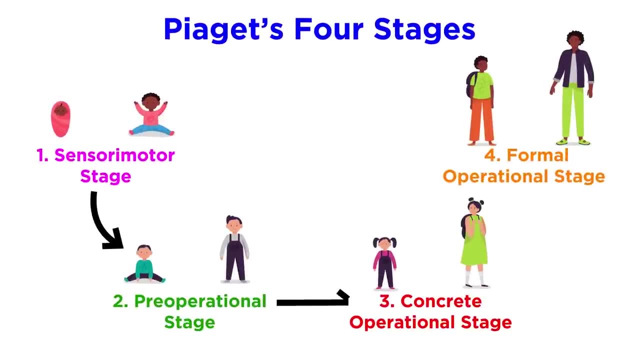 one quantity is increased. what happens to the second quantity? Piaget's four stages help us understand how children develop cognitively across development. Importantly, Piaget didn't think that kids develop by simply adding more knowledge to their brains as they grow up. 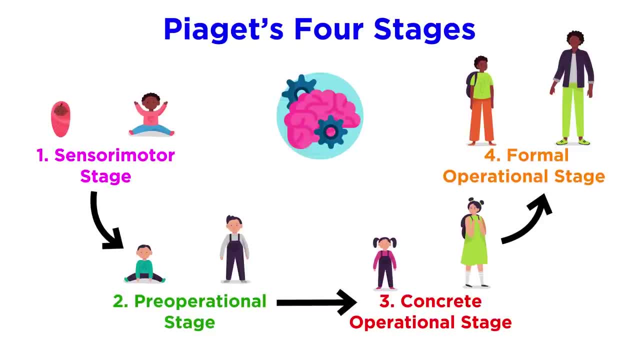 Instead, the quality of how they think is more important than how much knowledge they can gain from it changes as they progress through the stages. A seven-year-old thinks differently than they did at age two. Today, psychologists generally appreciate and accept Piaget's stages. 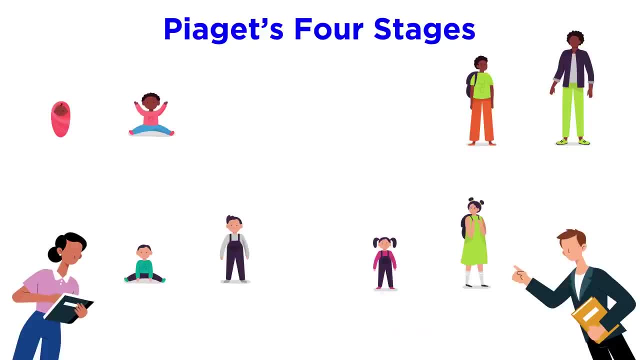 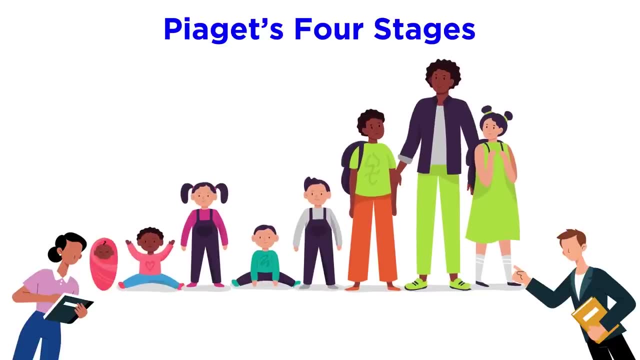 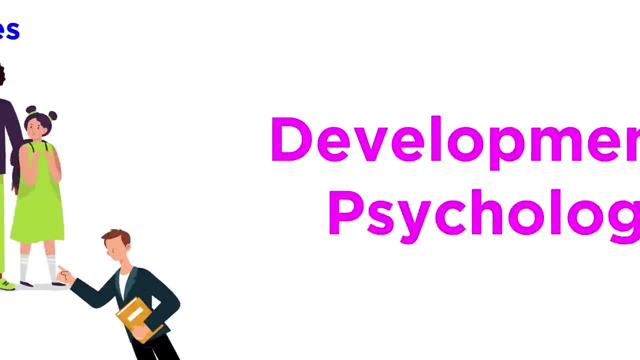 with some caveats. As we mentioned earlier, there is a lot of variation in how children develop. Not all children will move through these stages at the same times. Still, Piaget's stages provide a useful framework for thinking about child development, and they played a huge role in. 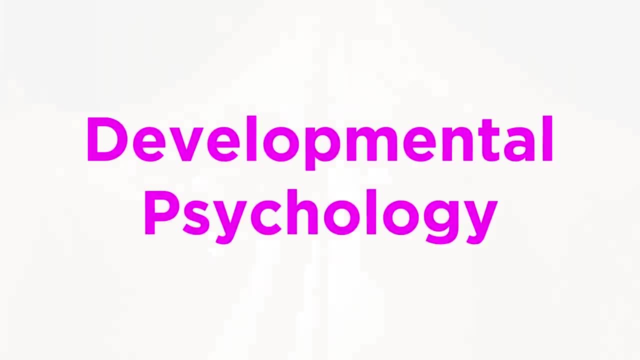 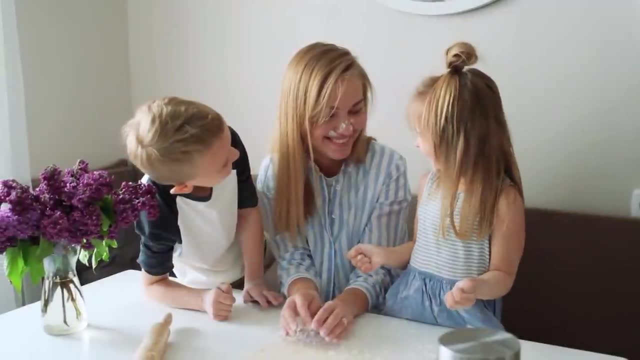 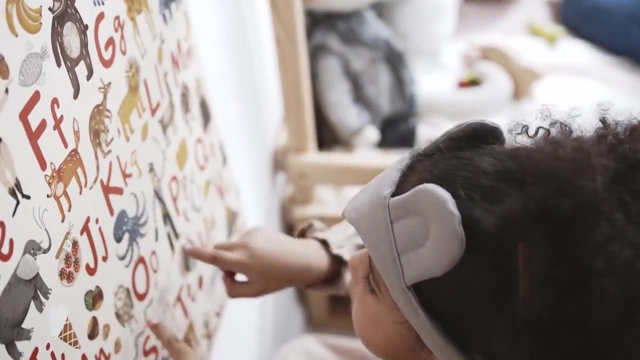 influencing the field of developmental psychology. His theory also helped psychologists realize that kids think differently than adults and that they aren't just smaller versions of adults. There's a lot more we could say about different topics in developmental psychology and perhaps later in the series we will go deeper with this fascinating subject. But for now 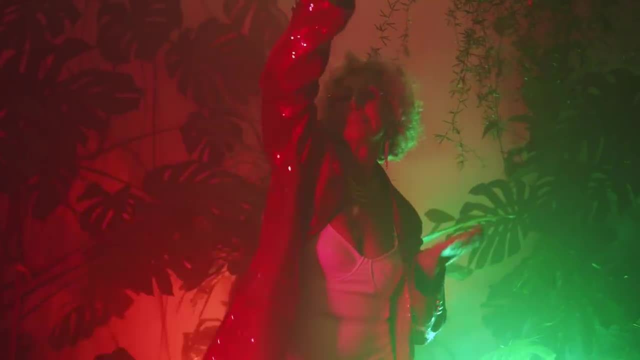 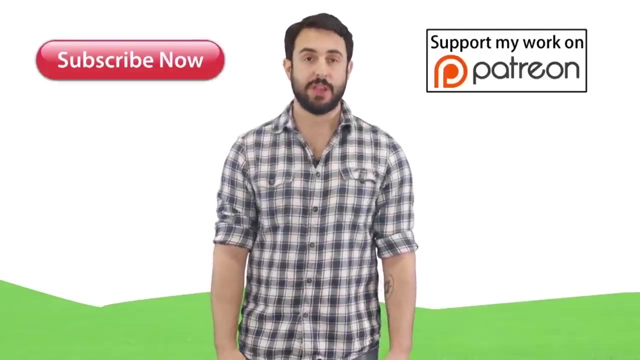 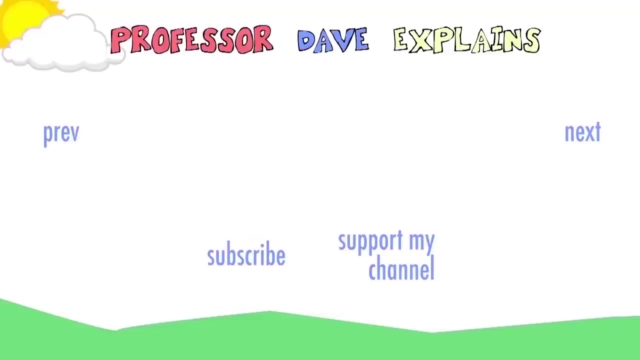 we're going to move on to the next topic in this series, which is the topic of the day. The topic of the day is the series Personality. The topic of the day is the series Personality. The topic of the day is the series Personality.